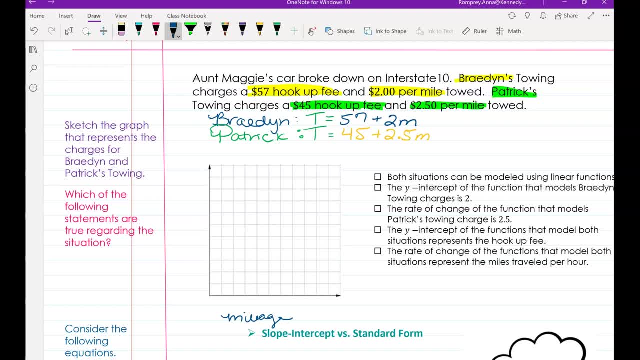 the X-axis where total charge is going to go on the Y-axis, Okay. So it's probably not super often that we're only going to get total total charge. All right, one mile, I mean maybe, but so maybe do like 5, 10, 15, 20, 25 miles. that seems like. 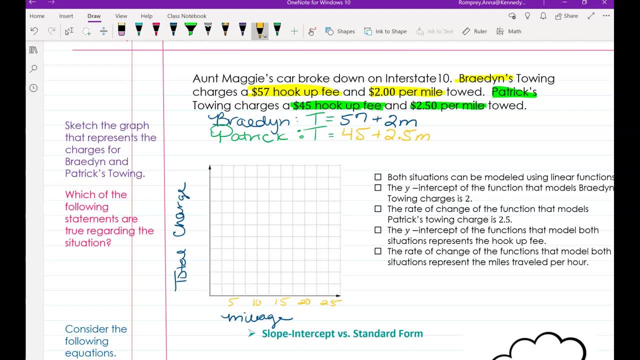 a lot. so the total charge. well, let's see we're starting at 57 and 45. so let's just put a break in the graph and let's see if we're going at 5 miles. so if I plug that in 2 times, 5 is 10, so 67. so we're jumping from 57 to 67 to 77, 87 if. 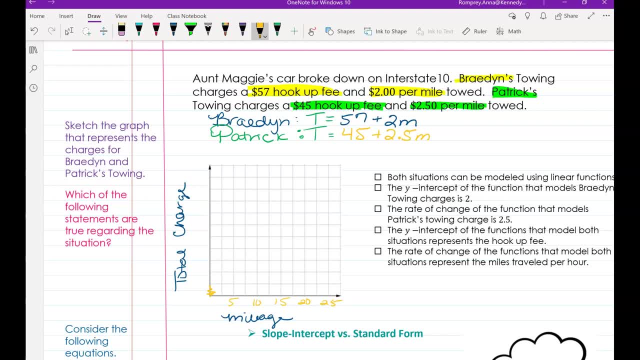 we keep that pattern going, okay, so we'll get up to around 100. so here: 250 a mile. so for 5 miles gives me increases of 1250. so 45, okay. so 200 should be good, all right. so I'm gonna start at, I guess, 40 and I'll just buy. since we're going up by 10 and 1250, I'll. 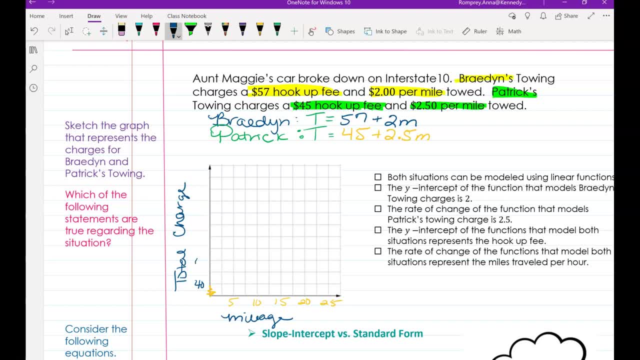 just number by tens. so 40, 50, 60, 80, 100, 120. I'm thinking that should get us started, okay. so again, Braden is starting at. okay, so I'll just make Braden blue. so Braden starting at 57. so about there. so 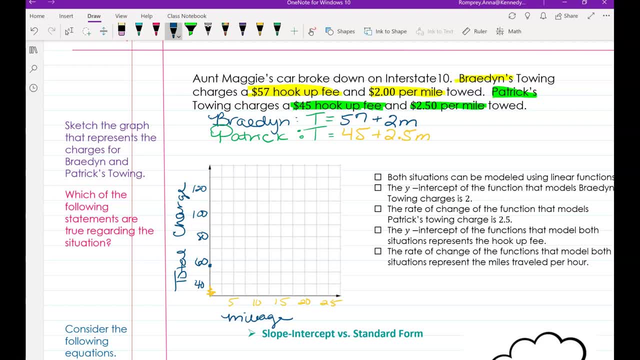 at 5 miles. I'm gonna add another. so 67, 77, 87. do you guys get what I'm doing? because I just did 2 times 5. so for every 5 miles we're going to increase by $10. so I'm just jumping. so 97, 107, all. 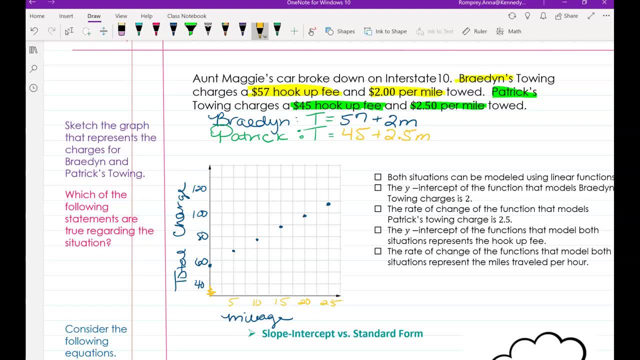 right, that's plenty. so then, Patrick only starts at 45, but is growing at 1250, so that's gonna go up to so 5, so 52, 50, and then sixty-five, seventy-seven, fifty, you, you, so 90, you, and then 102, 50. 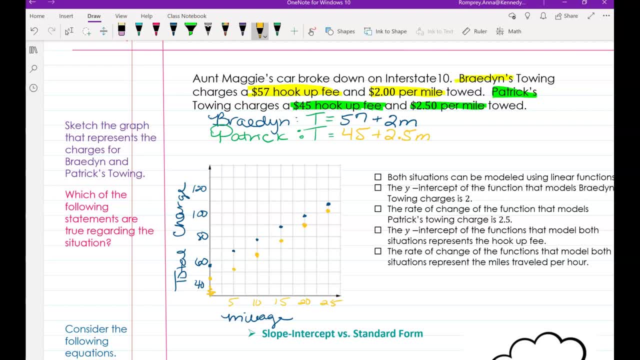 so gaining. so Patrick is definitely starting to gain on Braden. so Patrick looks at first Patrick is definitely gonna be cheaper. but once we go past a certain number, Patrick is gonna exceed Braden's cost. so it all depends on how has been many miles are you going. which company are you going to want to use? so both? 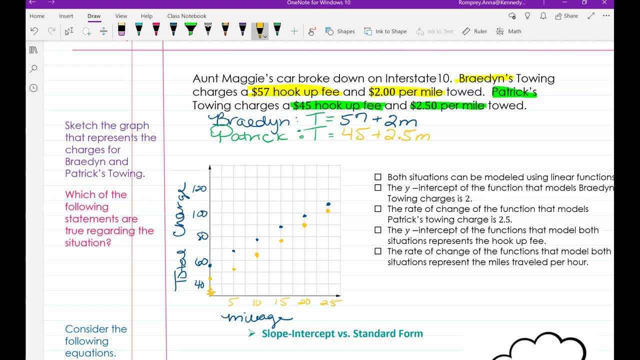 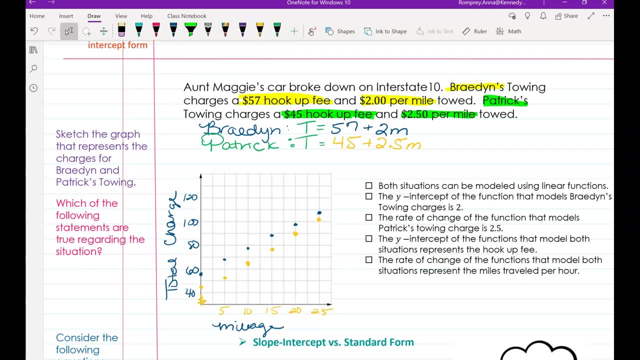 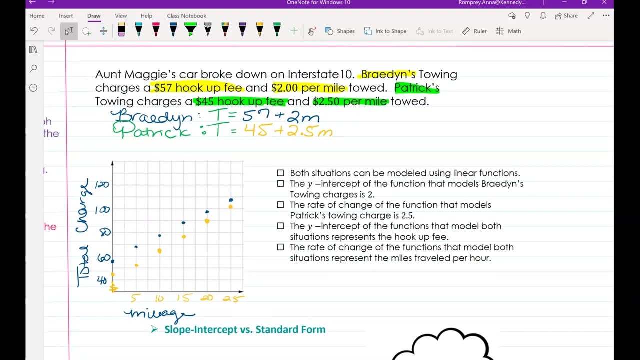 going. which of the following statements are true regarding the situation? ok, so depends on how many miles are you going. which company are you gonna want to use? is situations? it says which of the following statements are true regarding the: both situations can be modeled using linear functions. situations can be modeled using linear functions. yes, I'm increasing by ten each. 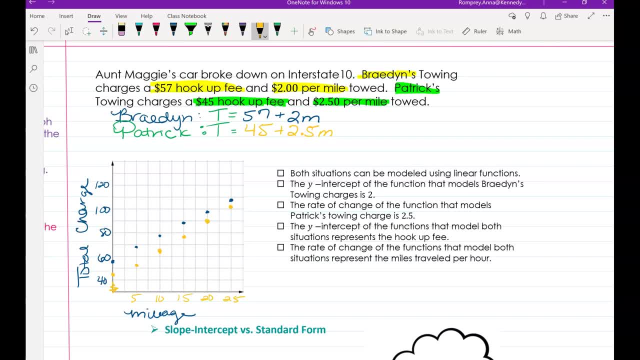 ten each time I have five miles and 1250 every time I have five miles. so that's a profit. buy 3: modified it right, okay, so no, it's true. trade-off now ב 58. that's a constant, constant rate of change. So, yes, both can be modeled using linear functions, All right. 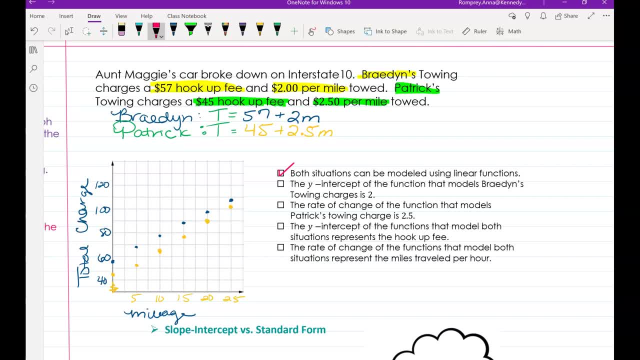 so the y-intercept of the function that models Brayden towing charge is 2.. So the y-intercept for Brayden? so over my y-axis that's definitely not 2.. Nope, it's actually 57.. Well, technically 0.57.. If you know, we should be precise. So the rate of change of the function. 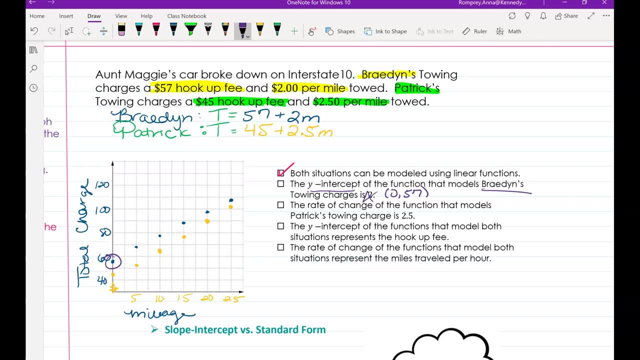 that models Patrick's towing is 2.5.. Well, let's see Patrick's towing rate of change: 2.5.. Yes, that's absolutely true. And the y-intercept of the functions that model both situations represent the hookup fee. 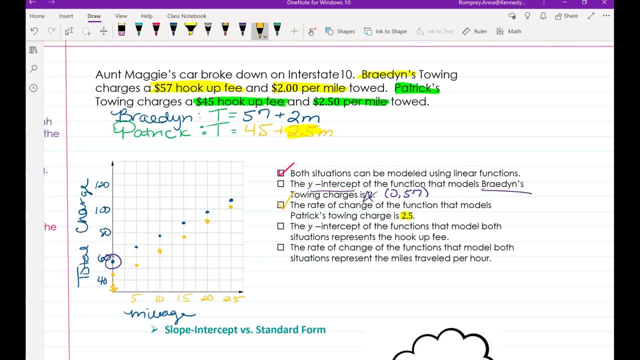 So the y-intercepts, that's where we're starting. whether we, even before they even drive us anywhere, just for showing up and hooking up the car, we have to pay. So the y-intercepts, yes, those are the hookup fee Check And the rate of change of the functions that model both situations. 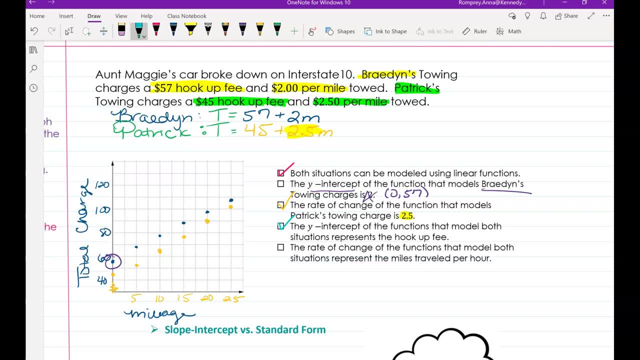 represents the miles traveled per hour. Okay, there's one little thing that messes that up, because m is for miles. yes, Miles traveled per hour. No, that's definitely not. It just represents the miles traveled. So if it just said miles traveled, that would be true, But they put in that per hour. Yeah, no, that's. 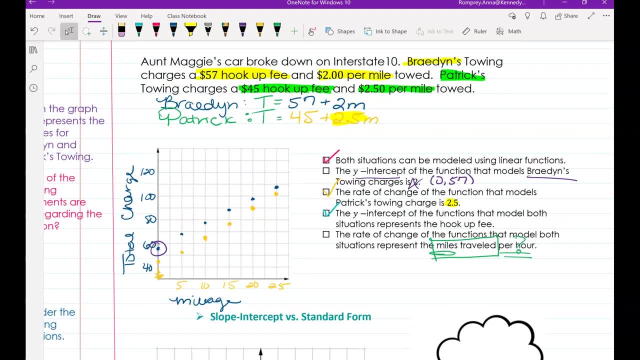 not right. So these are both linear models, Our hookup fee. so when you have an initial amount or initial fee that you're charged, that's going to be your y-intercepts And then from that y-intercept you're going to get the y-intercepts. So that's going to be your y-intercepts And then from that y-intercepts. 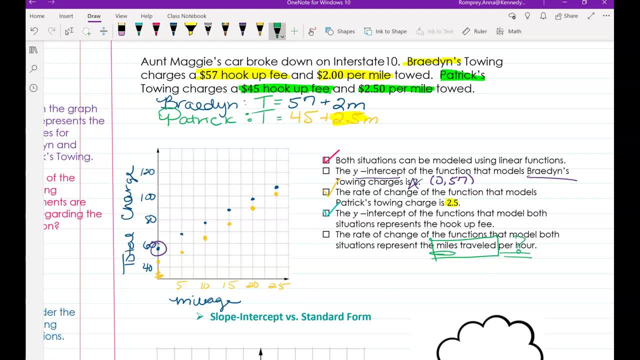 you're going to get the y-intercepts And then from that y-intercepts you're going to get the y-intercepts And then from that y-intercepts We're adding on, depending on what our rate of change is. So that just shows how much we either increase or decrease at a constant rate. 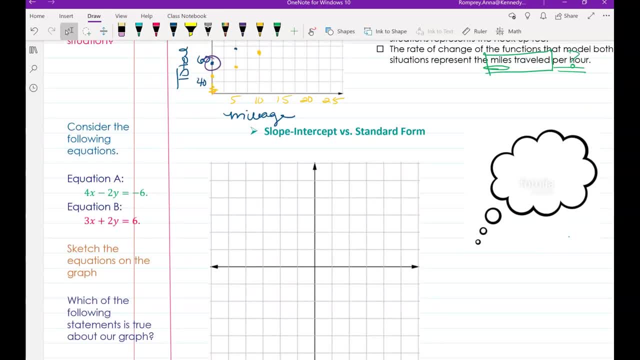 So let's look at, let's say we don't have a real-world problem and we're just given an equation. So it wants us to consider the following equation: So we're going to compare slope-intercept form versus standard form. So slope-intercept form, these might sound familiar. 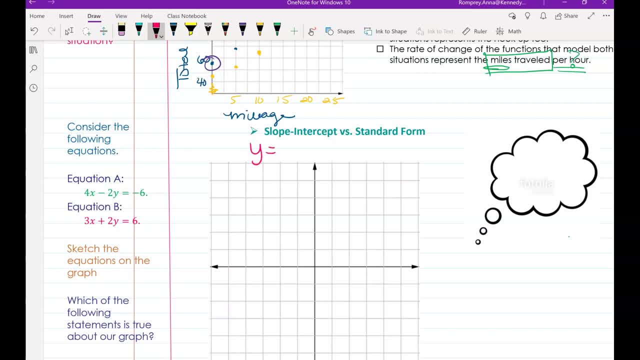 Slope-intercept form is y equals mx plus b, okay, Whereas standard form is ax plus by equals c. So notice, y is isolated in slope-intercept form. Standard form: ax plus by equals c. You just have your variables on one side and your constant on the other. 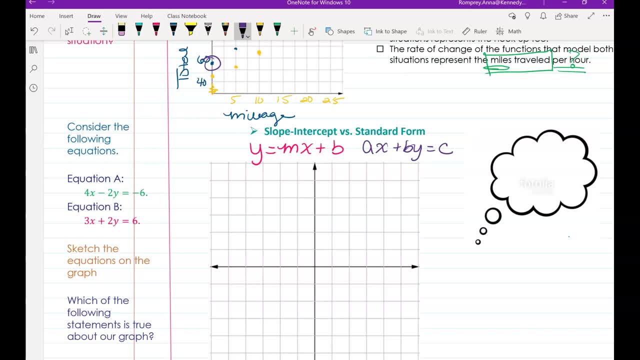 Okay, Standard form is very helpful for very little. Slope-intercept form we will use a lot. Before we move on, I want to dive a little bit deeper into slope-intercept form. okay, Because it really has so many useful pieces. 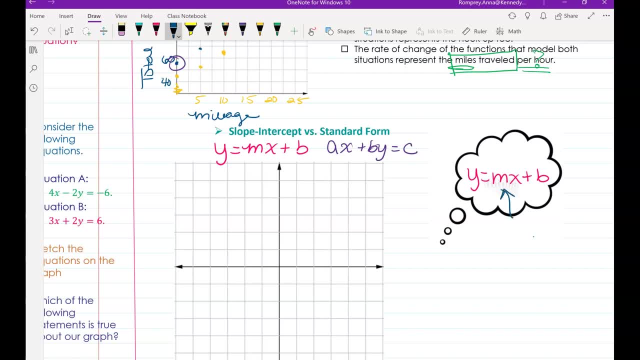 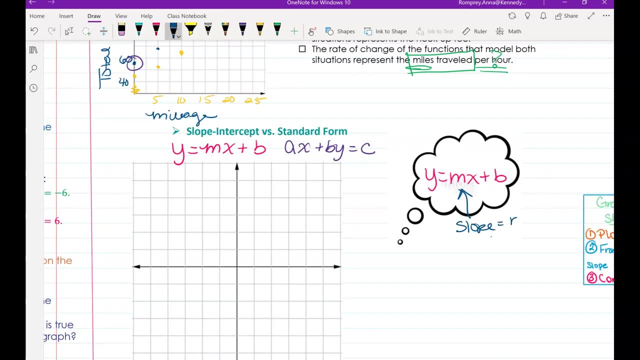 All right, so slope-intercept form m is our slope. So again, what's that phrase that we use for slope RISE OVER RUN? Okay, That's going to come in real handy when we're graphing. Now. b is a good starting point, all right? 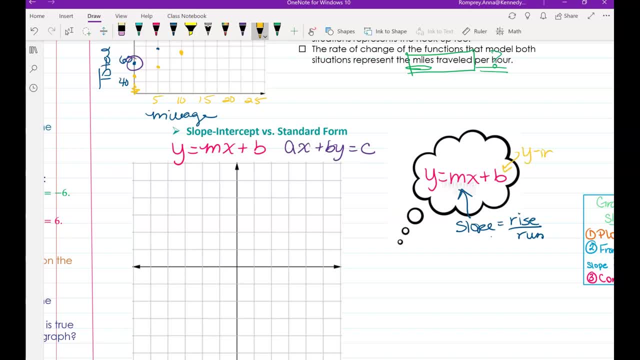 That is our y-intercept. So if b is positive, that means we have a positive y-intercept. If b is negative, we have a negative y-intercept. Okay, So I have got some steps over here. You can either pause this, but we're going to keep coming back to these. 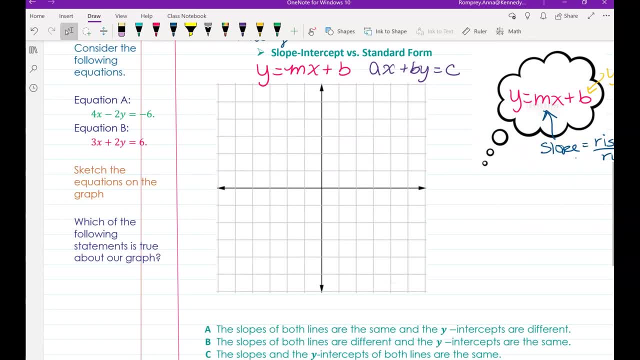 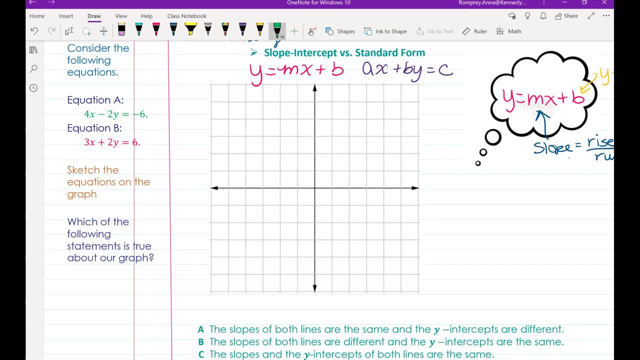 Anytime that we want to graph. okay, So let's go ahead and look at equation A. So equation A: 4x minus 2y equals negative 6.. All right, so that is in standard form. Standard form is not useful for graphing, but slope-intercept form surely is. 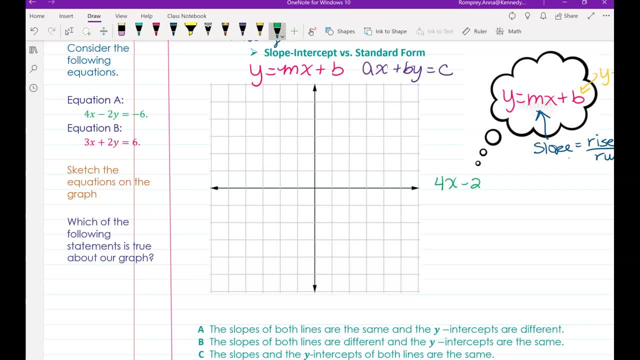 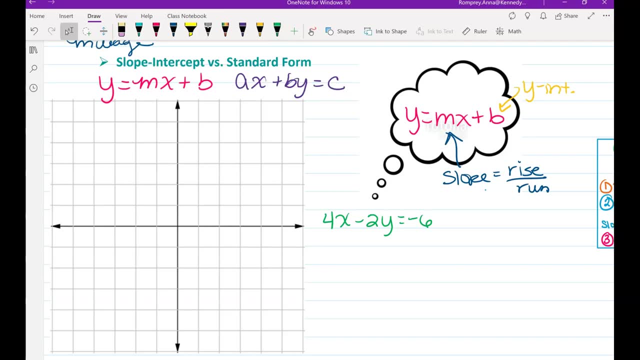 So I've got 4x minus 2y equals negative 6.. Okay, this is where that solving comes into play. Okay, The better you are at solving, the easier time you'll have with this. So I'm on slope-intercept form. so notice: y is isolated. 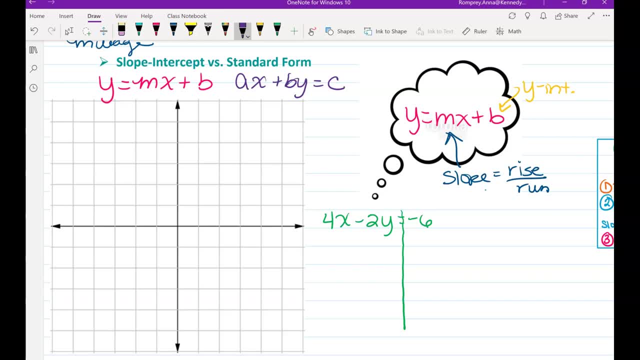 So I'm going to go ahead and isolate my y, So I'm going to move over my 4x first. so it's positive. So I'm going to take a negative 4x from both sides. So negative 2y equals. 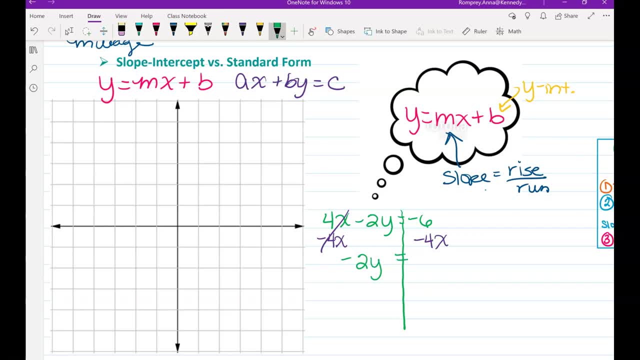 Now notice mx plus b. So I'm going to write the mx term first. So I'm going to write negative 4x first and then follow it by negative 6. It wouldn't be incorrect if you switch those. I'm just trying to write it in a way to where I end up in the proper format. 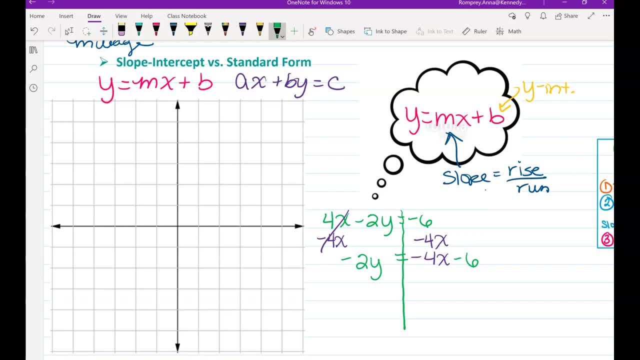 so I don't have to rearrange stuff at the end. Okay, so negative 2y or negative 2 times y. So I'm going to divide by negative 2.. So I need to divide all of my terms by negative 2.. 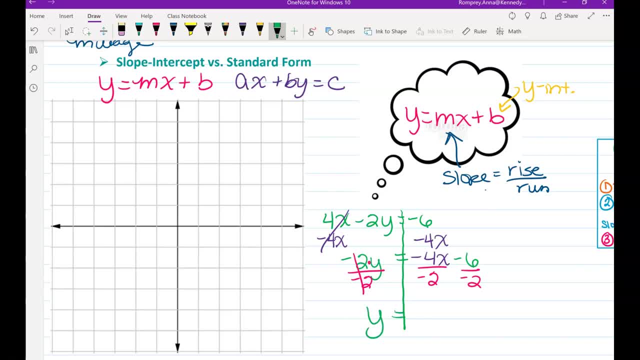 So y equals. So negative 4 divided by negative 2, that goes in evenly. So I end up with a positive 2x And then negative 6 divided by negative 2 plus 3.. So when we go to graph this, let's come over here and look. 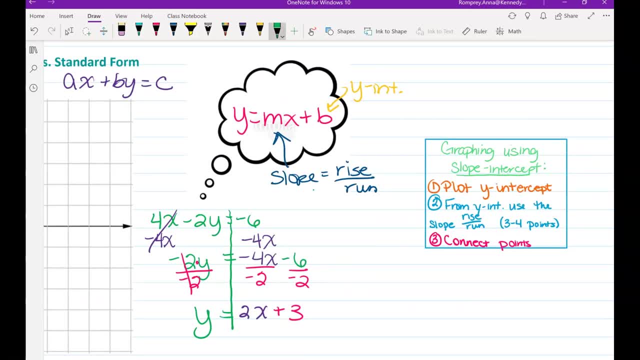 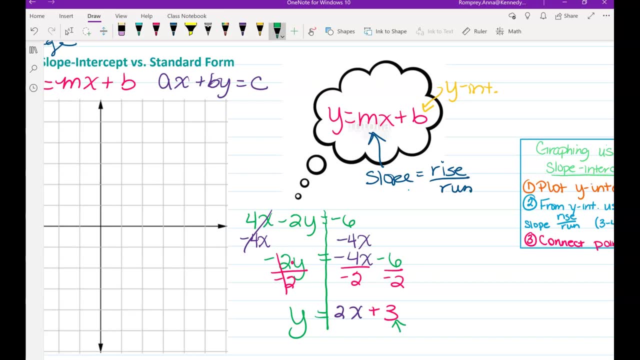 When graphing using slope-intercept form, first plot the y-intercept. So let's give ourselves a place to start. So our y-intercept: positive 3.. So I'm going to start at positive 3.. And from positive 3, I'm going to use my slope. 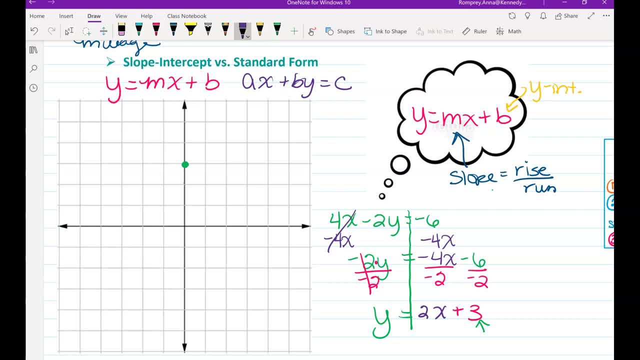 Now, slope is rise Over run. Well, I see a rise but I have no run. So what can I put this over? that won't change the quantity. Well, I can divide anything by 1. It doesn't change it. 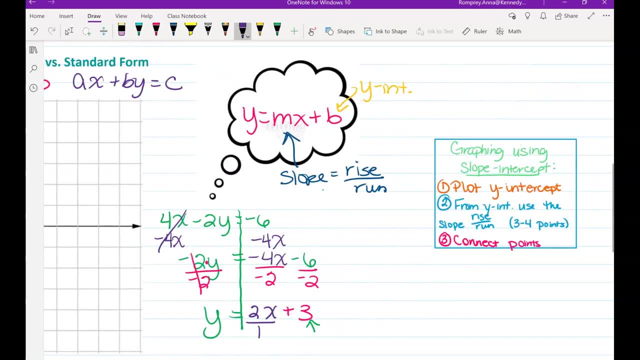 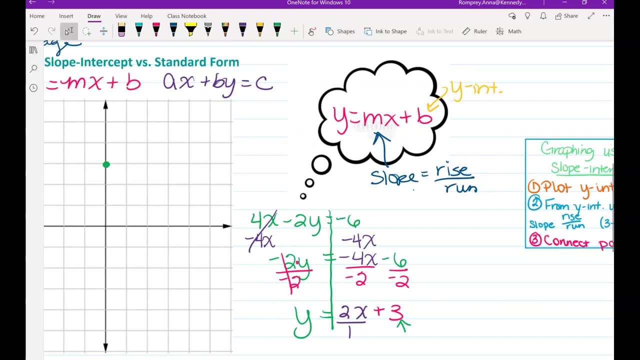 So 2 over 1.. So from your y-intercept, from your y-intercept, use the slope Rise over point, Rise over run, Sorry, And we'll try and get 3 to 4 points so we have something nice to connect. 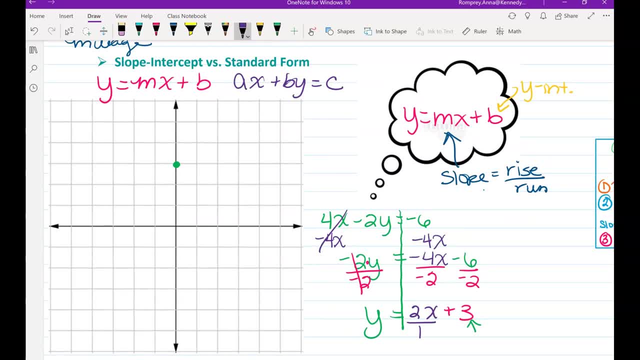 So my rise over run is positive 2 over 1.. Positive 2 over 1.. No, That was wrong. I ran 2 instead of up. So Oh no, So I ran out of room on my graph. So since I can't rise 2 and run 1 anymore, I'm going to come back to that point. 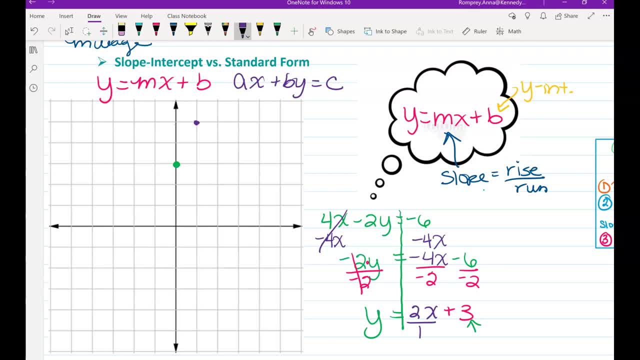 I'm going to do the exact opposite, so they stay in the line. So now I'm going to go down 2. And left 1.. Notice, I'm still in line. I just want a couple more points: down 2,, right 1.. 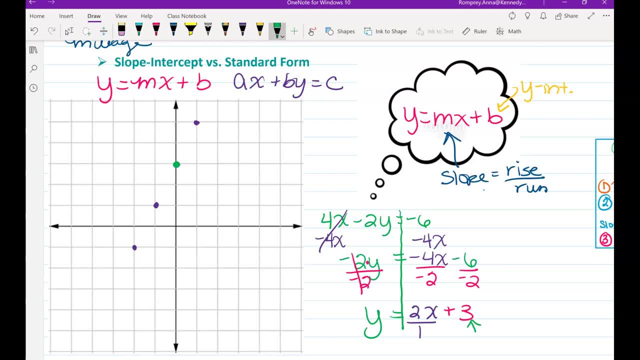 Sorry, left 1.. And now we can connect our points. Now I have something that's shaping up to be a line, So I'm going to connect Beautiful, Okay. So I would recommend that you go ahead and pause the video. 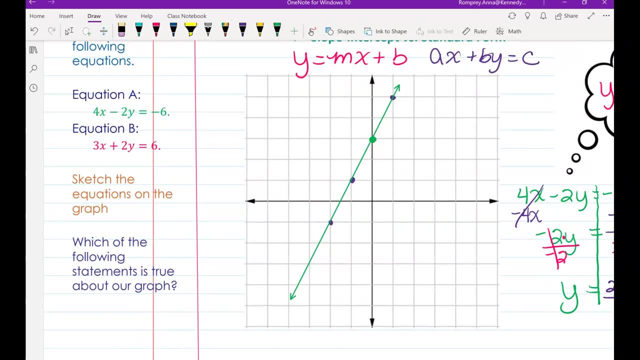 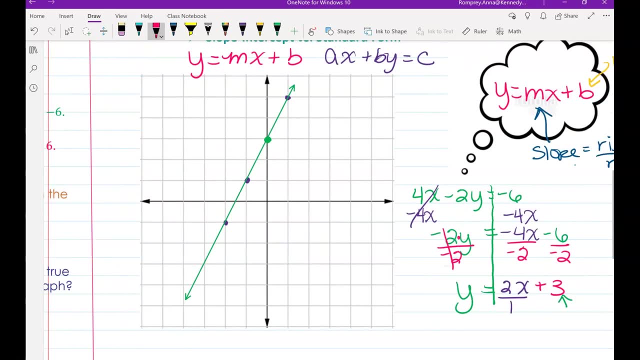 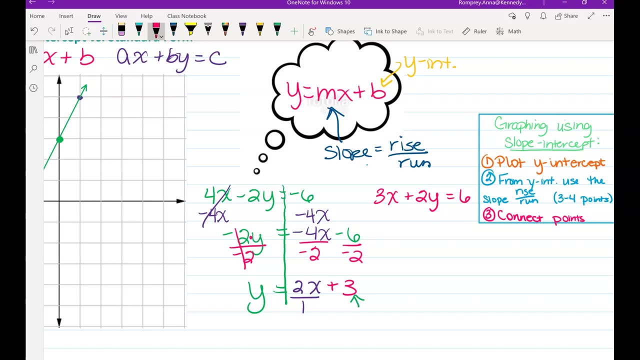 And try and do: 3x Plus 2y equals 6.. Try and do that yourself, Okay, And then, when you're ready, come back and check your answer, Alrighty. So I'm going to go ahead and put this in slope intercept form. 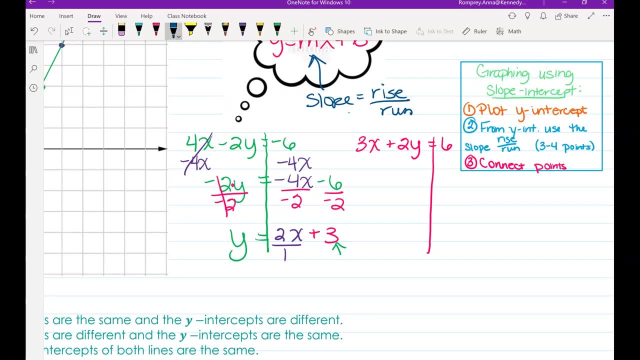 So I'm going to isolate my 2y. So first thing, Subtract 3x, Subtract 3x, So I have 2y equals. I'm going to write my mx first. So negative 3x plus 6.. 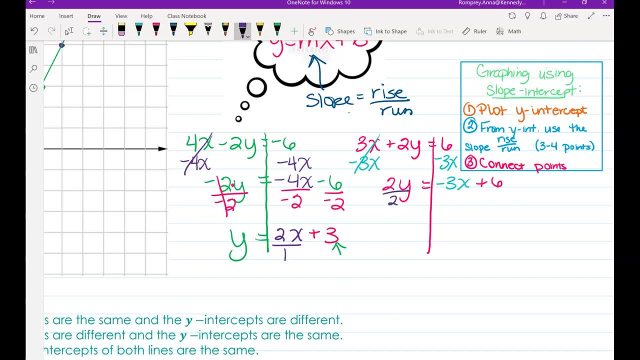 And I'm going to divide all of my terms by 2.. So y equals negative 3 halves x, Or you can write negative 3x over 2.. Remember that same thing, And then plus 3.. Alright, So let's try it out. 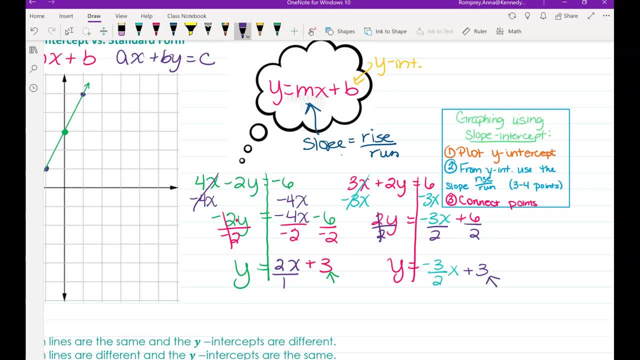 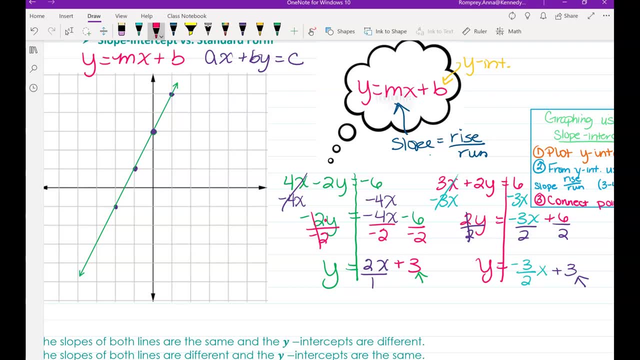 Again, where do we begin? I have a y intercept of positive 3.. Hey, that's what we had last time. Alright, So apparently our graphs are going to overlap, So from here I am going to use my slope, So our slope. 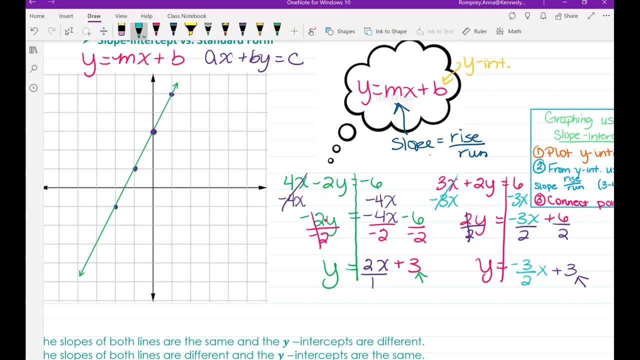 Negative, 3.. So from this point I go down 3. And then positive 2.. So right, 2. Down, 3.. Right, 2.. Okay, And I'm going to have one over here. So I'm going to come back and I'm going to do the exact opposite. 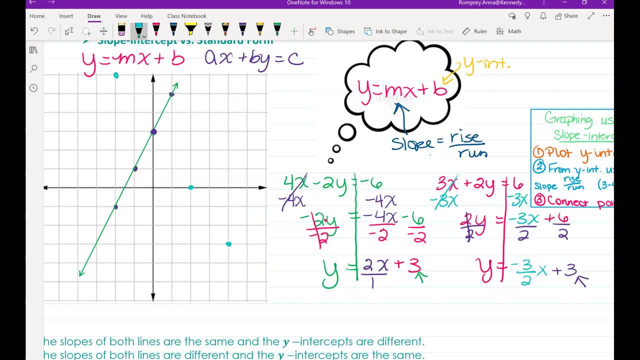 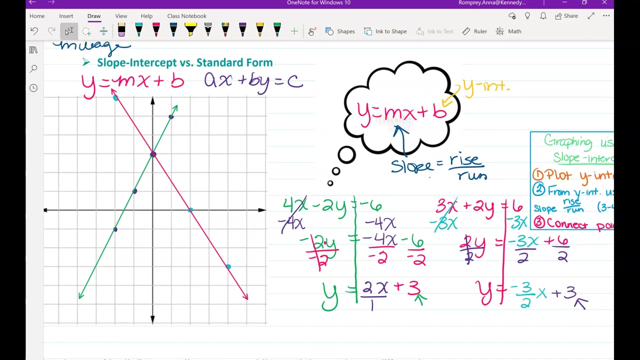 Up 3. And left 2.. So I've got plenty of points, So I'm going to connect. So come up here And beautiful. So even though I color coded my lines, if you're ever putting more than one line- well, really more than one graph at all- on the same coordinate plane, you technically should always label them. 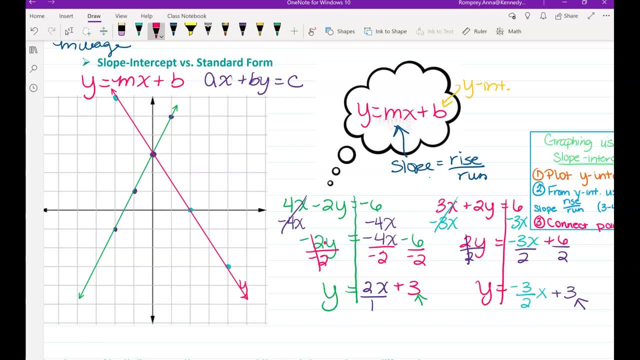 So this is y equals negative 3 halves x plus 3.. And this one is y equals 2x plus 3.. So I mean, technically, If you're color coding and I know what you're talking about, I'm okay. 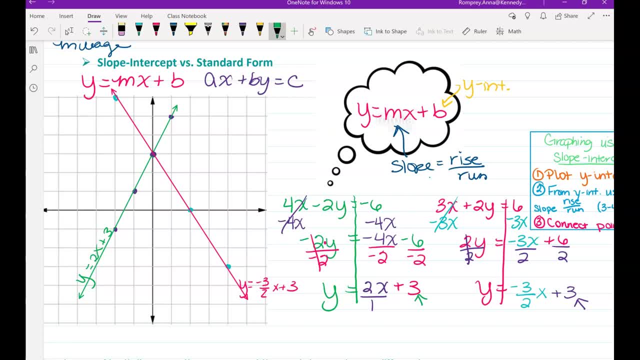 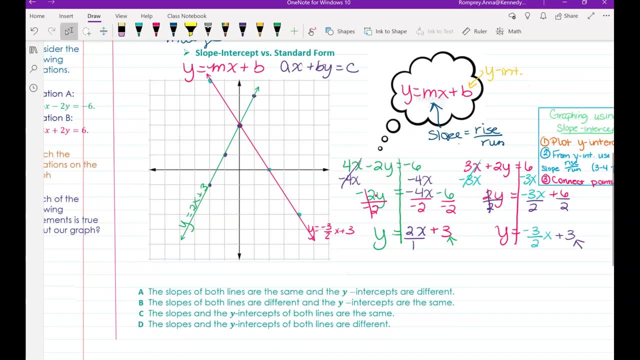 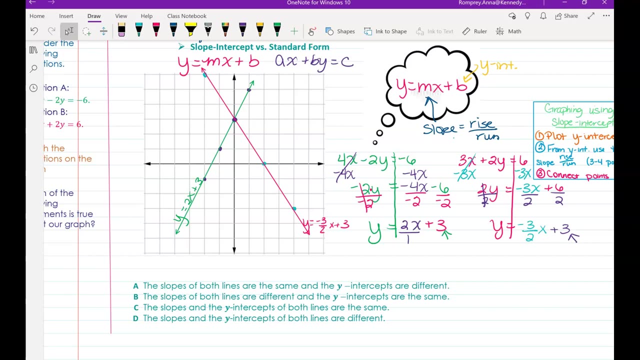 But again, if we want to keep our math correct, that's really how you should demonstrate it. One last piece. It says which of the following statements is true about our graph: Okay, The slopes of both lines are the same and the y-intercepts are different.